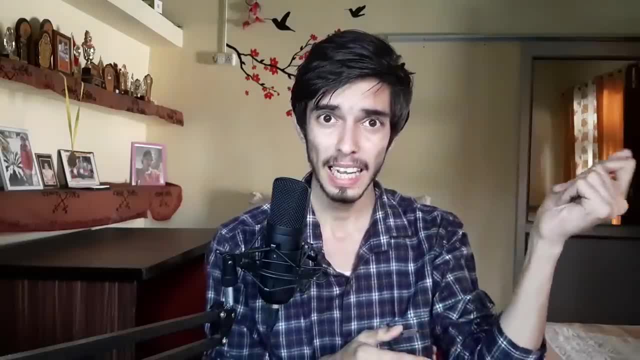 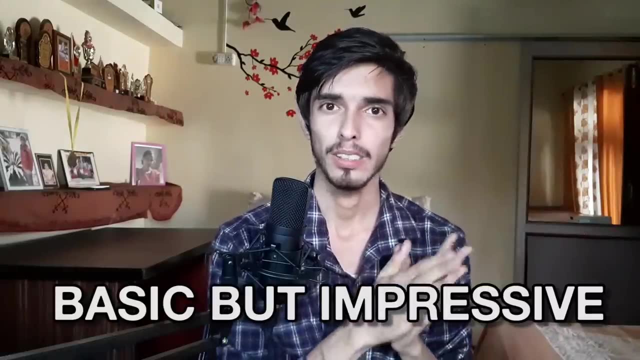 you how to do lightning fast calculations in snap, and which will amaze your friends and also help you academically a lot. So let's start with one of the most basic but really impressive math trick. This trick is also really famous, so I guess most of you will already know it, but let me teach you. 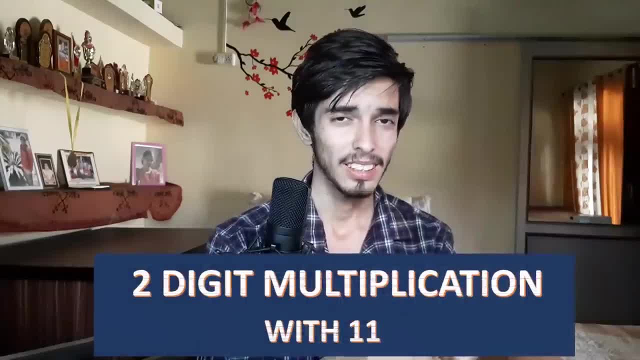 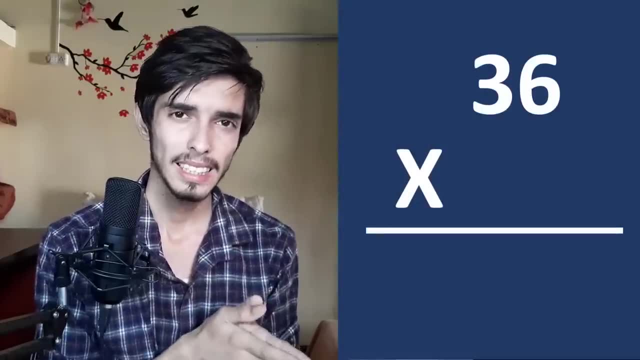 that first. So the trick is 2 digit multiplication with 11.. This is a really basic trick. So let's take an example. How would you multiply 36 by 11?? Now, if you solve it with the method you learn in, 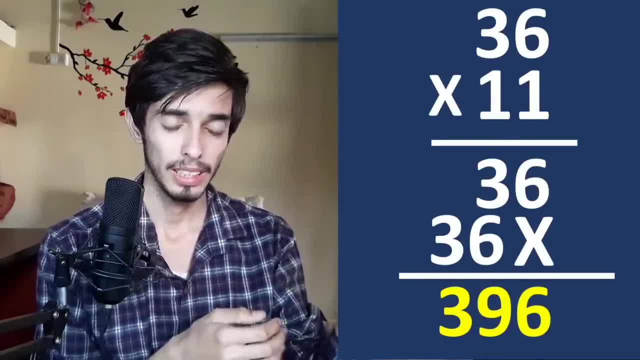 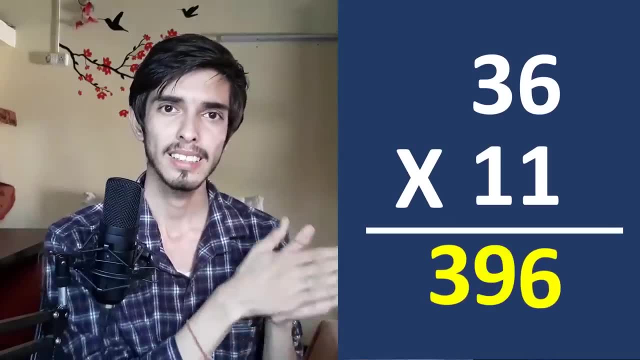 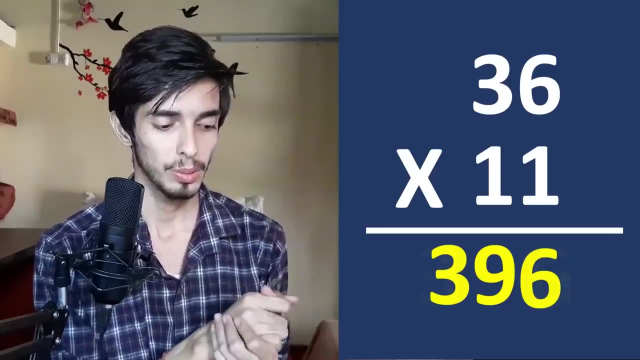 school, then this problem is easy, but a little longer. But if you use this trick like write 3 and 6 and in the center add these two numbers, that is 396, which is the answer. See, lightning fast. Yeah, this is really basic, but yeah, this is a cool trick too, So let us try. 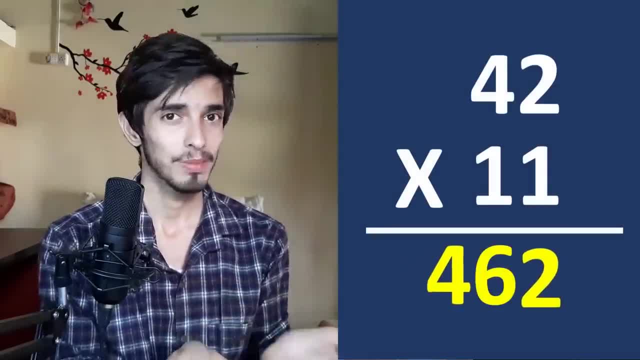 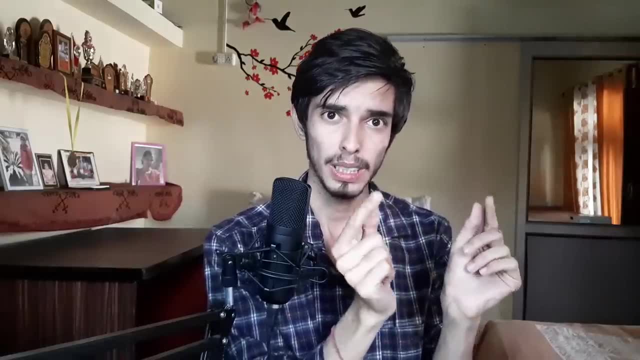 another 42 multiply by 11, which is 462.. As fast as that. See in here you are faster than a calculator. Now you will say: this trick will only work if these two numbers add up to 9.. If they add up to, 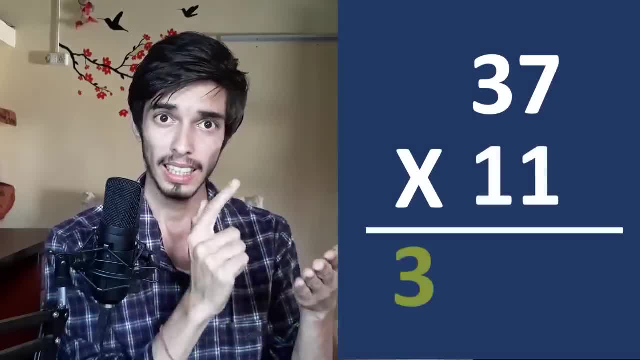 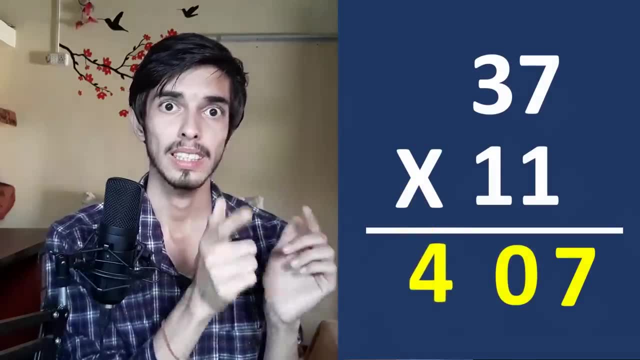 11,. what will happen then? So 3, and at the end it is 7, and 7 plus 3 is 10.. So that 1 goes on to carry, So 407.. This is our answer. So this is how fast you can do it Now if you are really new in. 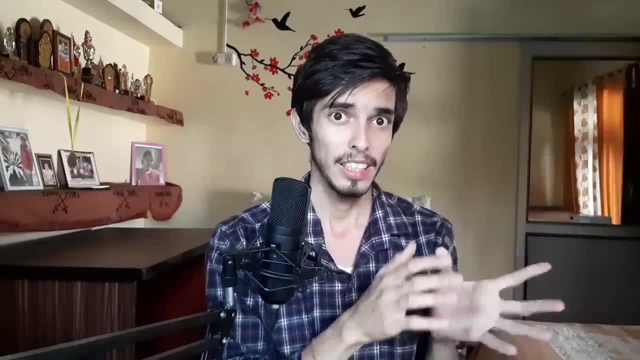 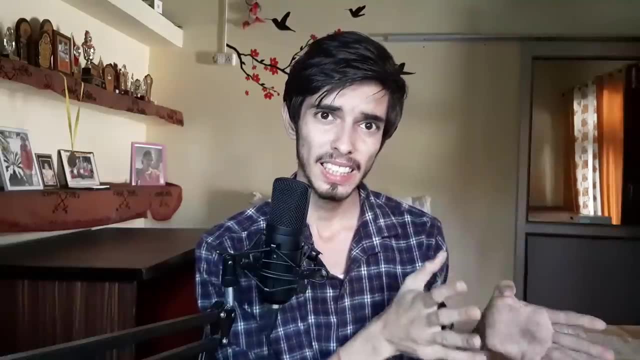 mental math. I know you will have a little problem in taking this carry, But trust me, as you go on this series, this will be a piece of cake for you. Now you know what you are thinking. You will say that you are just sharing tricks for specific number which will only work like for 11.. 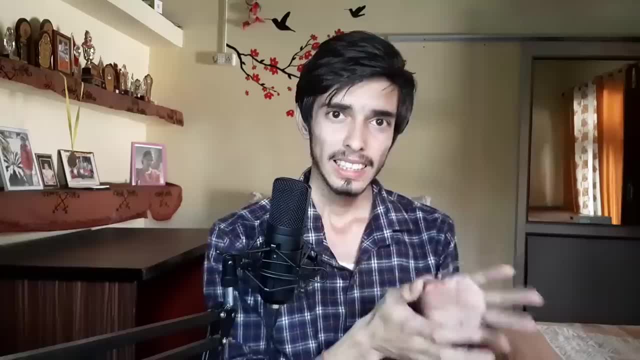 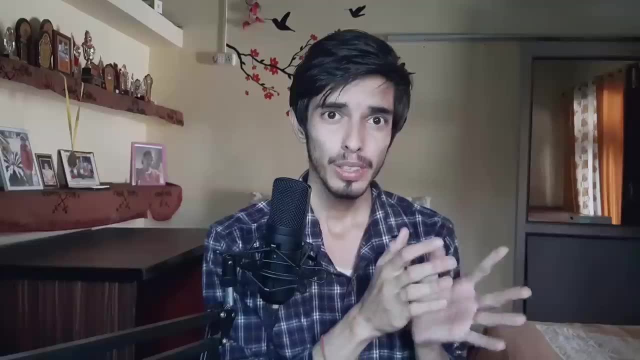 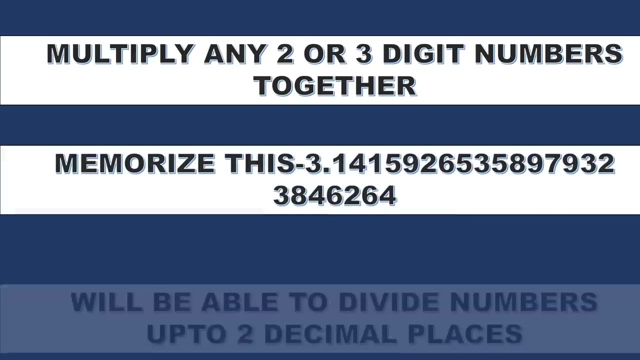 And for other numbers. This is not mental math. Yes, in this video I am just teaching some basic tricks to you, because this is the first part, But as we move on to this course, you will learn how to multiply two 3-digit numbers. You will be able to memorize the first 24 digits of pi. You will be 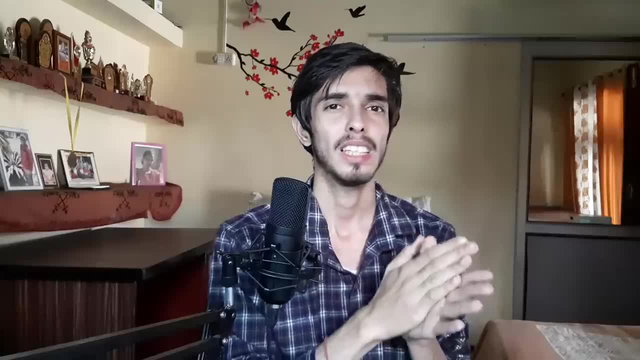 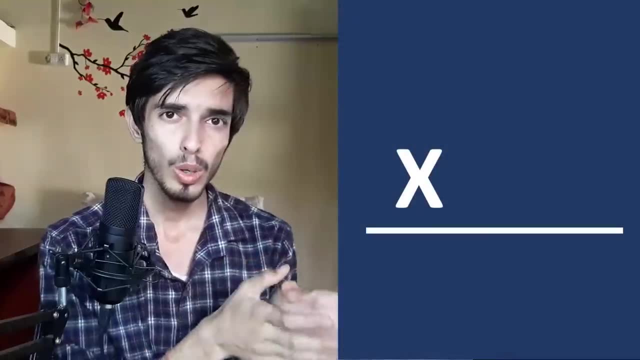 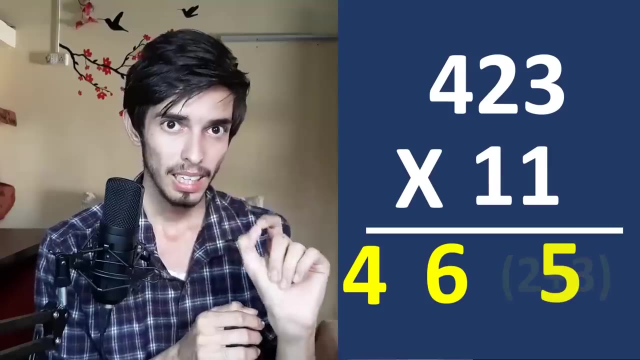 able to divide 2-digit numbers up to 2 decimal places and a lot more. Now the trick that I have taught you also works with 3-digit numbers: multiply by 11.. So let us take an example: 4, 4 plus 2, 6, 2 plus 3, 5 and 3.. This is our answer. Also, if there are carries, you just take. 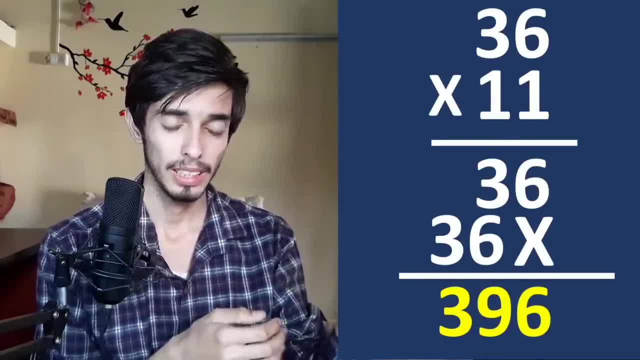 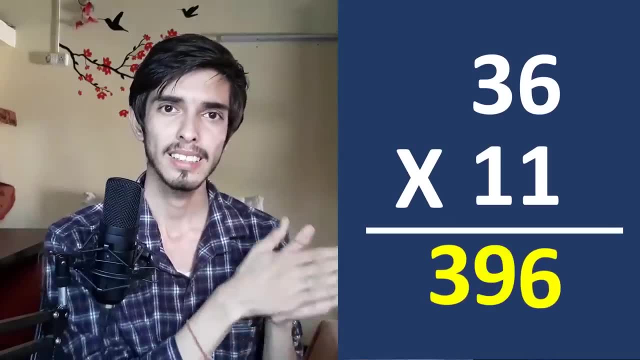 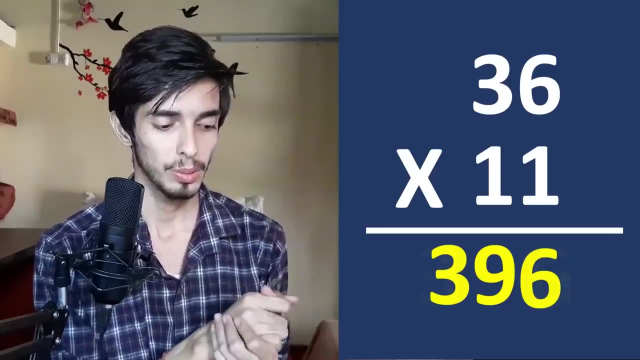 school, then this problem is easy, but a little longer. But if you use this trick like write 3 and 6 and in the center add these two numbers, that is 396, which is the answer. See, lightning fast. Yeah, this is really basic, but yeah, this is a cool trick too, So let us try. 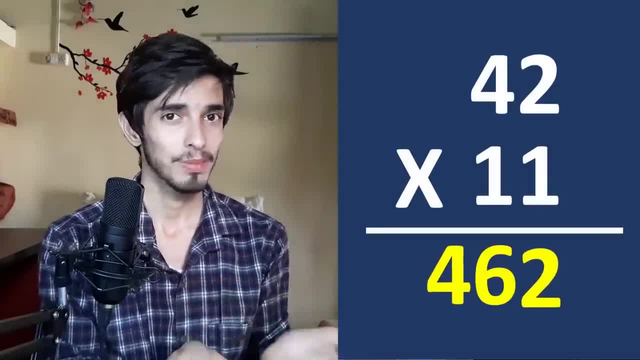 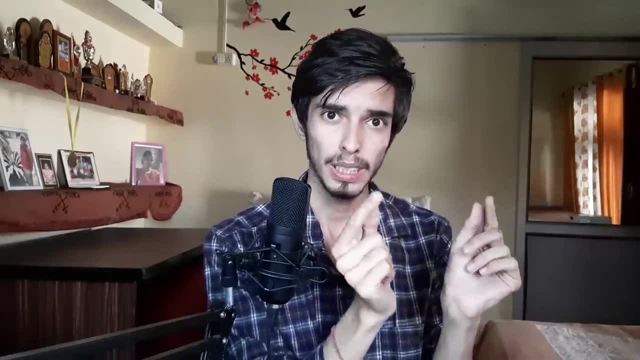 another 42 multiply by 11,, which is 462.. As fast as that. See in here you are faster than a calculator. Now you will say: this trick will only work if these two numbers add up to 9.. If they add: 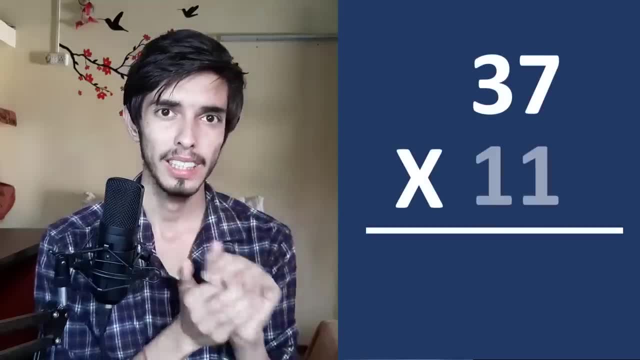 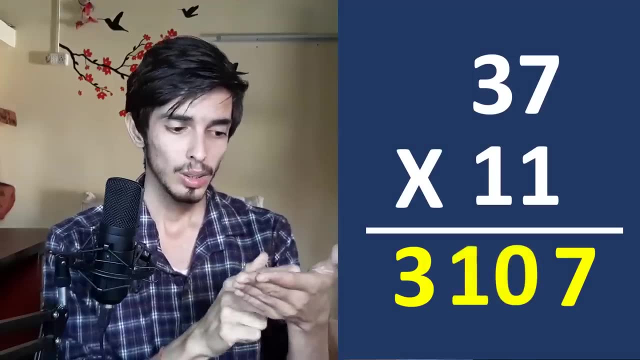 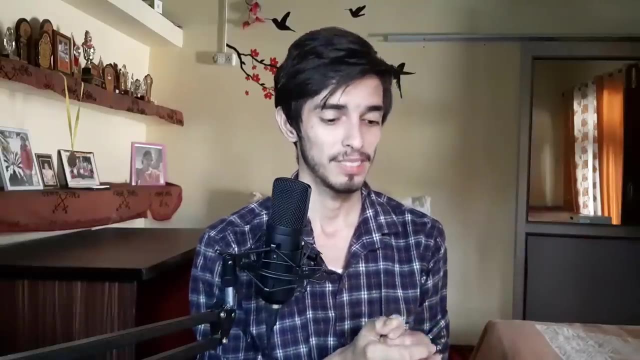 up to 10,. what will happen then? So let us do 37.. 41 multiply by 11, what will happen then? So 3, and at the end it is 7, and 7 plus 3 is 10.. So that 1 goes on to carry, So 407.. This is our answer. So this is how fast you can do it. 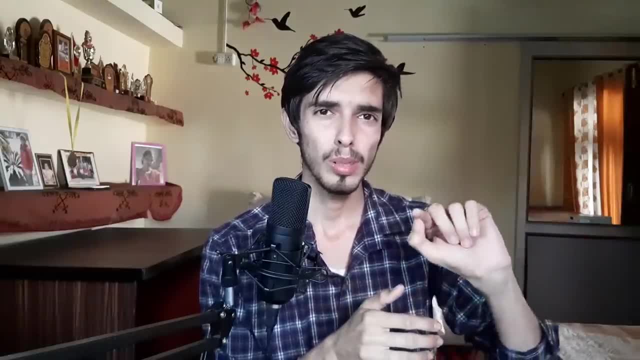 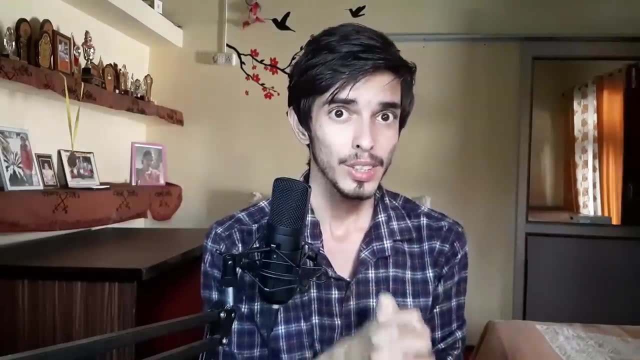 Now, if you are really new in mental math, I know you will have a little problem in taking this carry, But trust me, as you go on this series, this will be a piece of cake for you. Now you know what you are thinking. You will say that you are just sharing tricks for specific number which will only work, like for 11.. 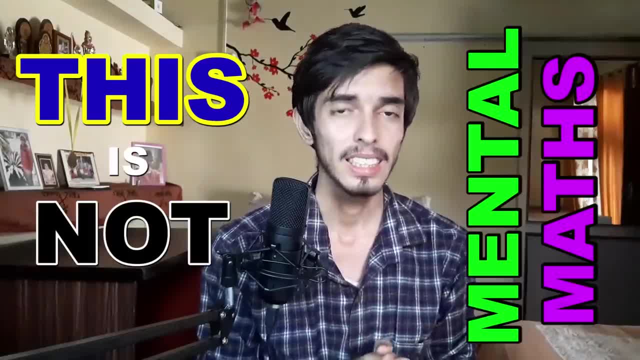 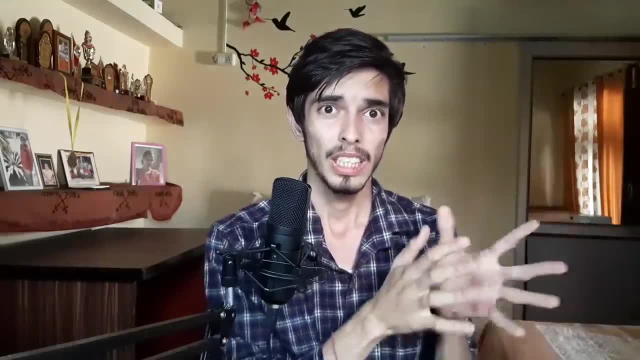 7 and 4 other numbers. This is not mental math. Yes, in this video I am just teaching some basic tricks to you, because this is the first part, But as we move on to this course, you will learn how to multiply two 3-digit numbers. You will be able to memorize the. 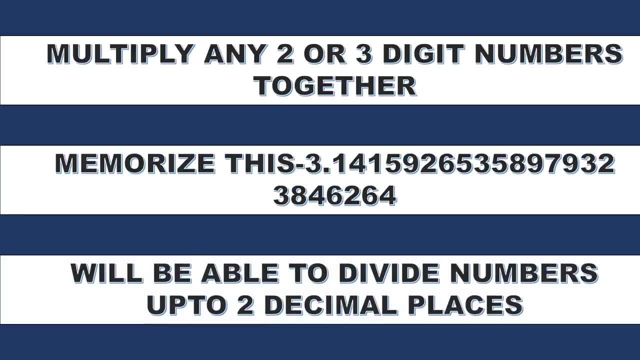 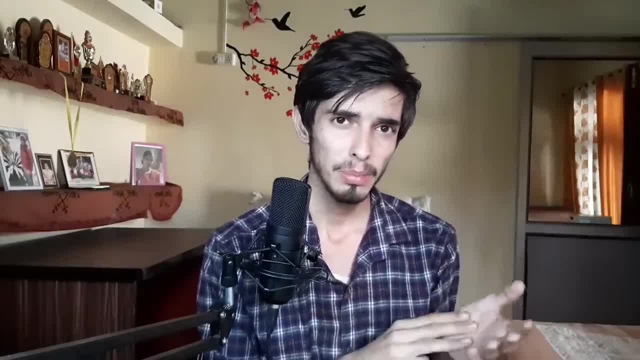 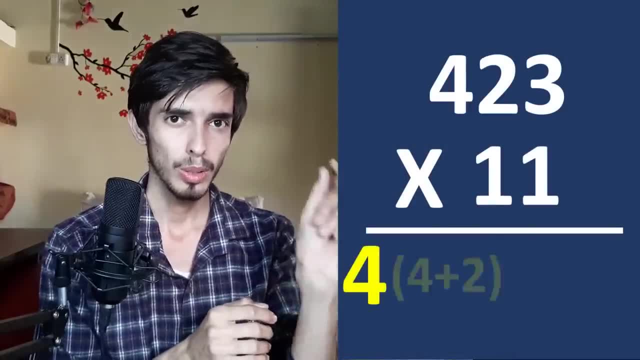 first 24 digits of Pi, You will be able to divide 2-digit numbers up to 2 decimal places and a lot more. Now the trick that I have taught you also works with 3-digit numbers: multiply by 11.. So let's take an example: 423 multiply by 11.. So 4, 4 plus 2, 6, 2 plus 3,. 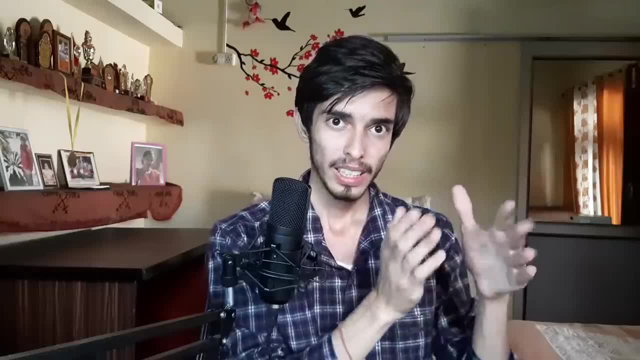 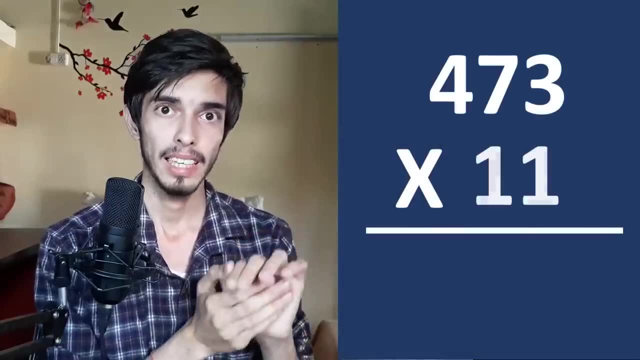 5 and 3.. This is our answer. Also, if there are carries, you just take the carry, like we have done in the previous problem. So let's take an example: 473 multiply by 11.. So see: 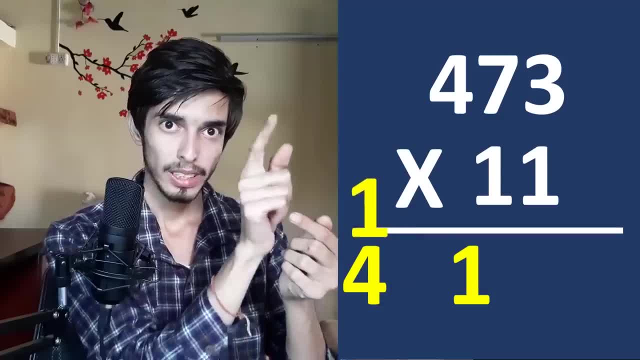 4 and 7 plus 4 is 11.. So 4 will change into 5.. So 5, 1 and 7 plus 3 is 11. So 4 will change into 5.. So 5, 1 and 7 plus 3 is 11.. So 4 will change into 5. So. 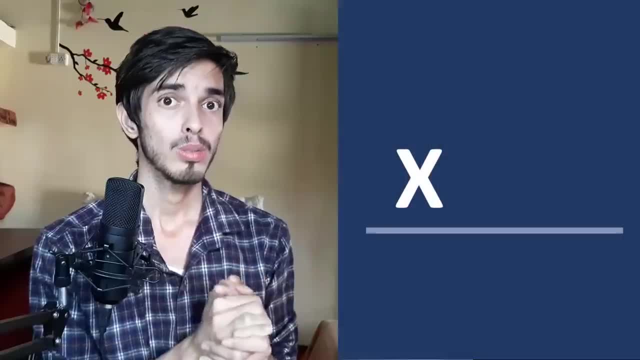 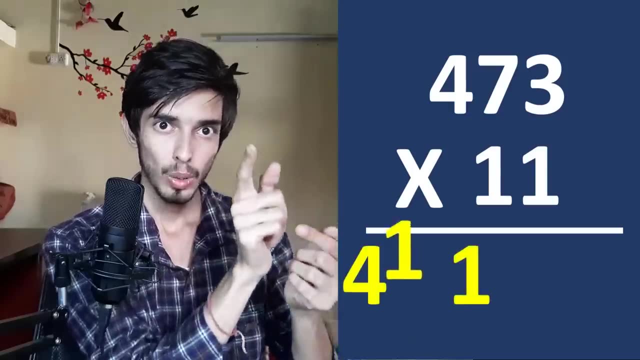 the carry, like we have done in the previous problem. So let us take an example: 473 multiply by 11.. So see 4 and 7 plus 4 is 11. So 4 will change into 5.. So 5, 1 and 7 plus 3 is 10. So. 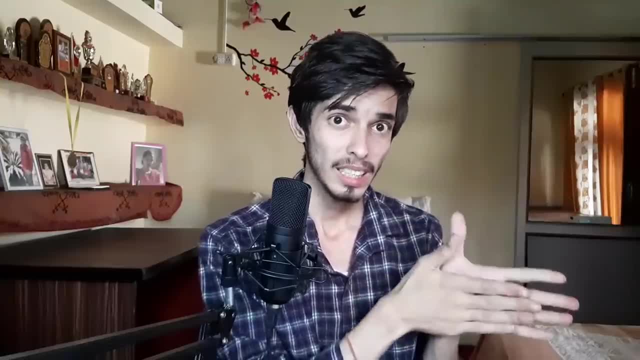 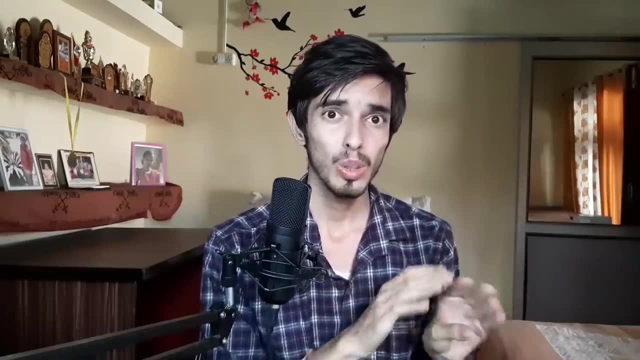 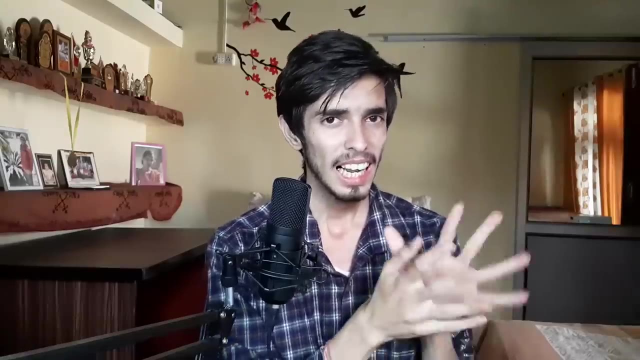 this is our answer. As simple as that. See, you are here, also faster than a calculator. So just after these two tricks, you are able to multiply any 2-digit number or any 3-digit number by 11.. So this is how cool mental math is. So now let us take it to a next level. I have a question for. 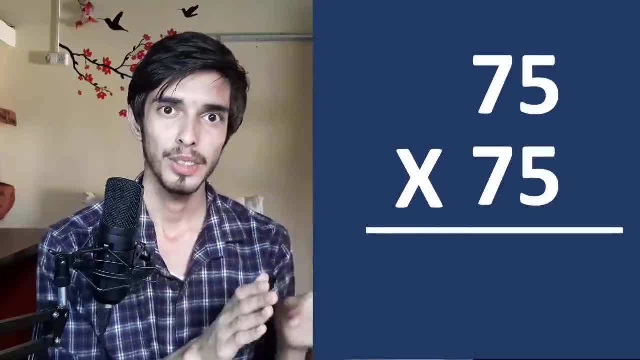 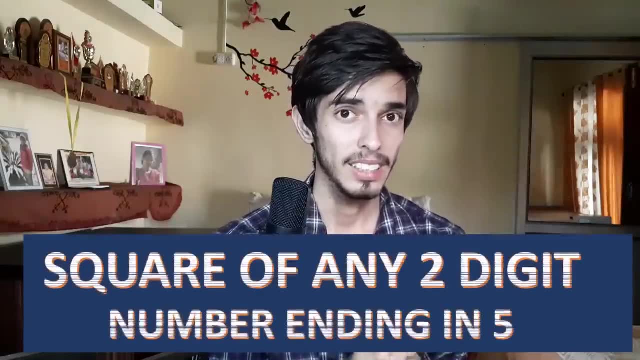 you Multiply 75 by 75 in your head right now and note that time. So our second trick is multiplying 75 by 75. So now you have just multiplied 75 into 75 in your head and I guess it would be really. 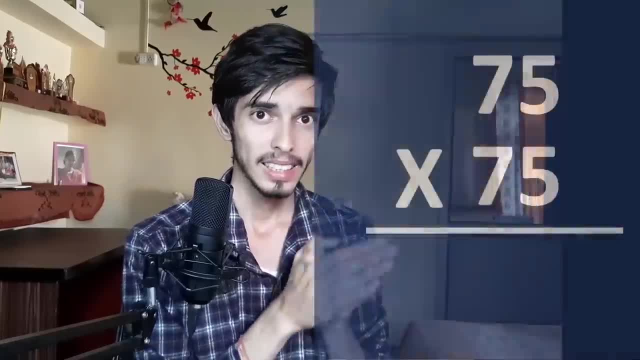 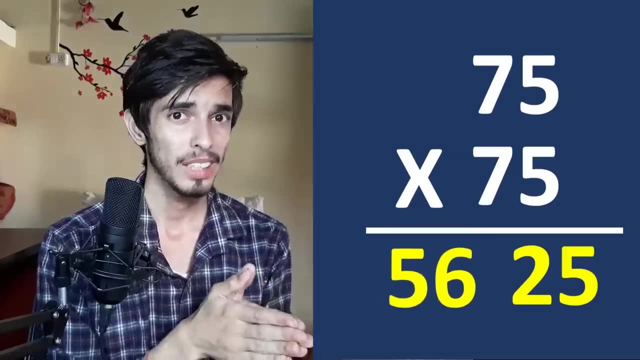 difficult for you if you do not know this trick, And the trick is that multiply 7 by its next number. like 7, 8 is a 56 and the answer ends in 25.. So 5, 6, 2, 5 is our answer. As simple as. 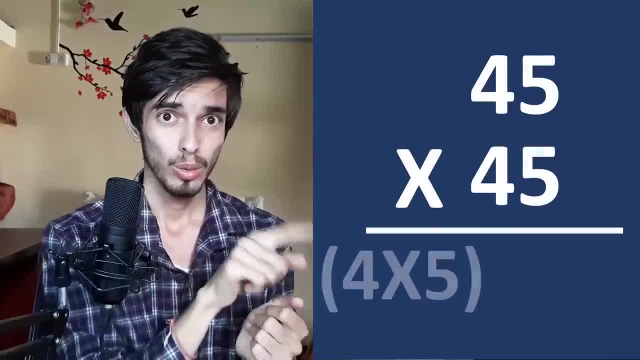 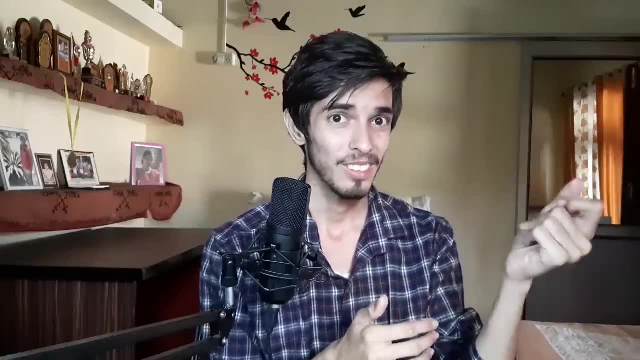 that. Let us take some other examples: 45 into 45. So 4, 5 is a 20.. 2, 0,, 2, 5. 15 multiply by 15.. 1, 2 is a 2.. 2, 25.. As simple as that. See, we are faster than a calculator. So let us take 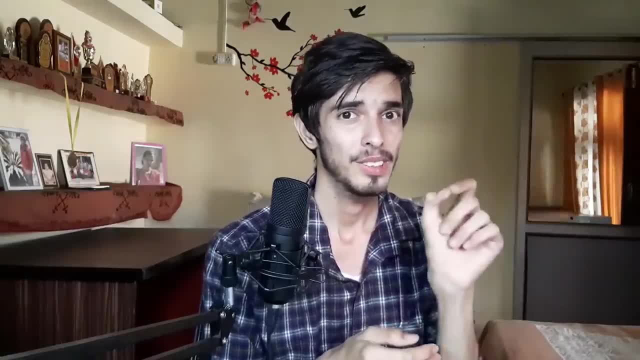 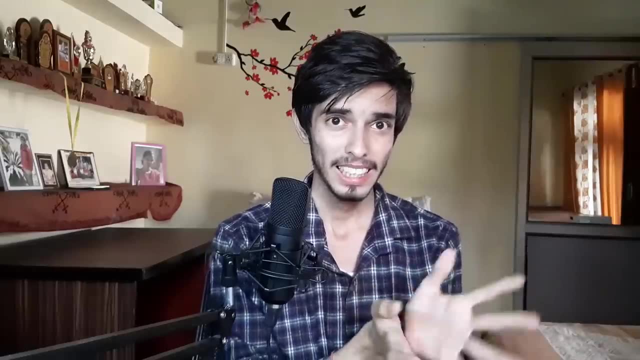 a calculator in here also. I just want to tell you that I have added this 75 into 75 problem in my game, MathLobran, And people were like how will we do it in 3 seconds? But here we are doing it in. 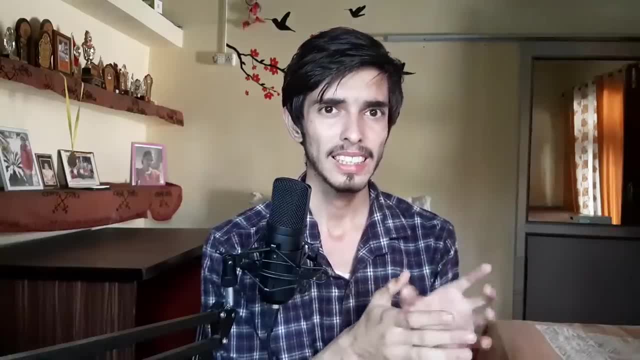 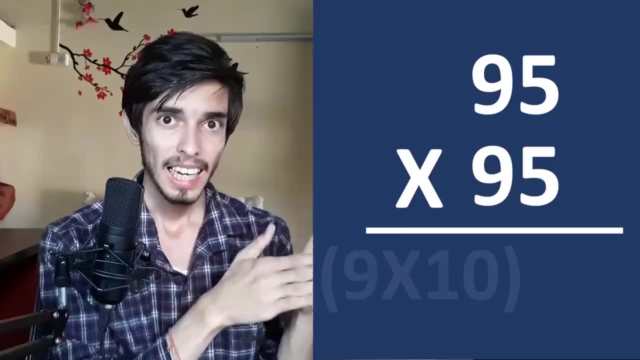 1 second Now. the biggest number you can do with this trick is 95 into 95.. That is 95 square. So the answer is you tell Yes, 9 into 10,, 90, 25.. As simple as that. We have just done it in a snap. 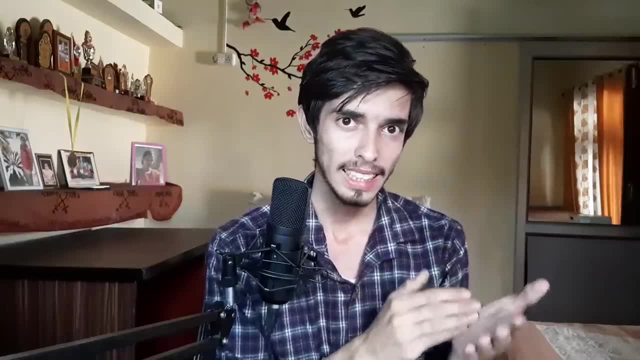 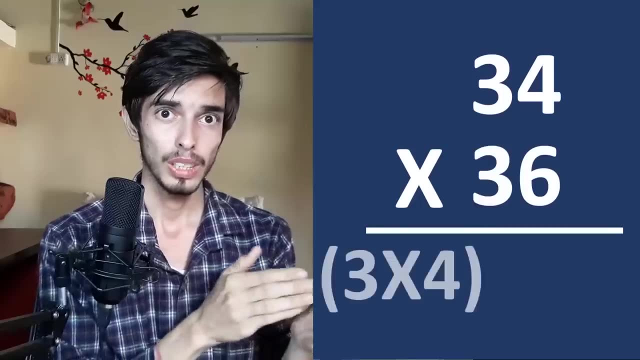 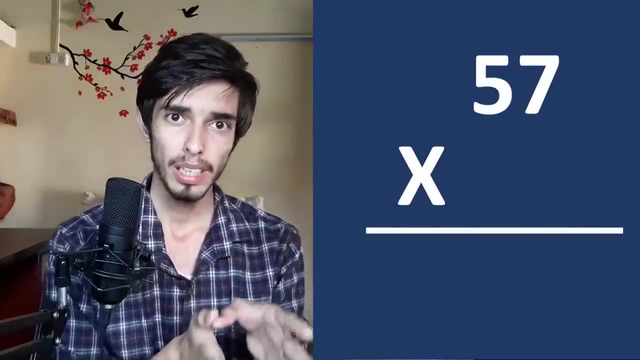 Now, this same trick also works with numbers which have same starting digit and the ending digits are adding to 10.. For example, 34 multiply by 36.. 4 is a 12 and 6, 4 is a 24.. 12, 24 is our answer. So now let us take another example: 57 multiply by 53. 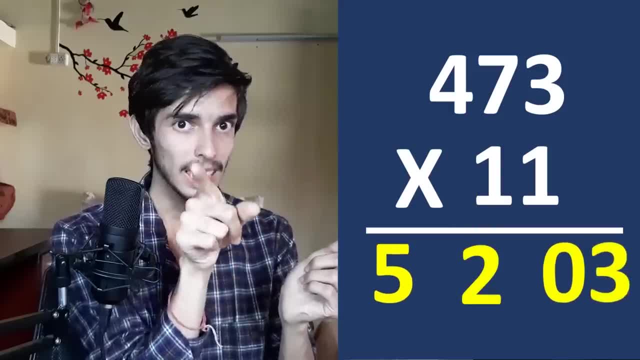 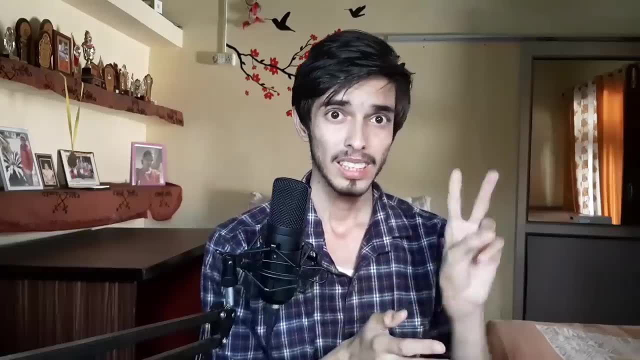 10. So 5,, 2,, 0,, 3.. This is our answer. As simple as that. See, you are here, also faster than a calculator. So just after these two tricks, you are able to multiply any 2-digit. 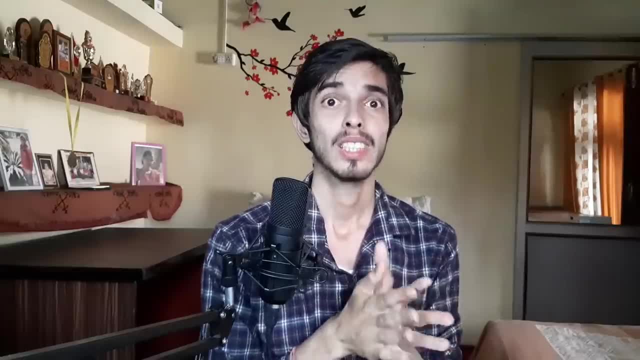 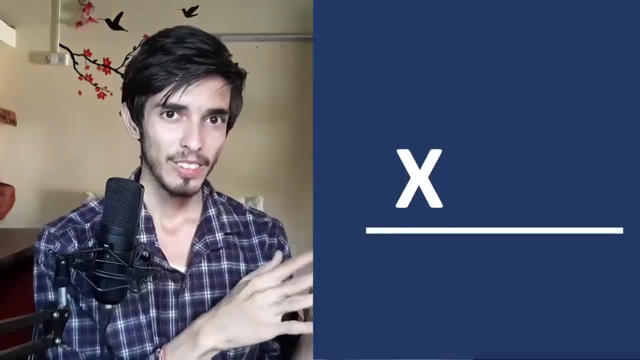 number, or any 3-digit number by 11.. So this is how cool mental math is. So now let's take it to a next level. I have a question for you. Multiply 75 by 75 in your head, right? 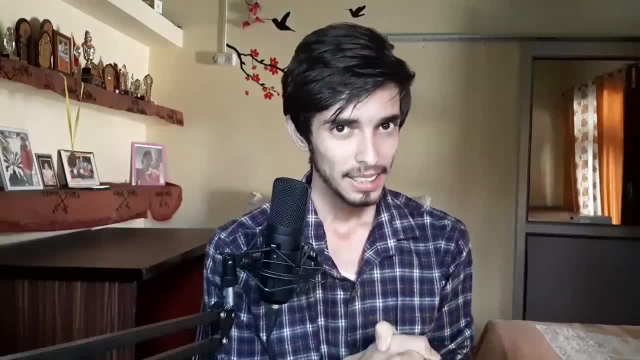 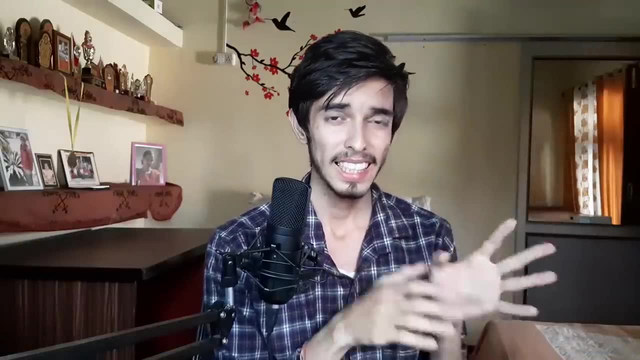 now and note that time. So our second trick is multiplying any 2-digit number ending in 5.. So now you have just multiplied 75 into 75 in your head and I guess it would be really difficult for you if you don't know. 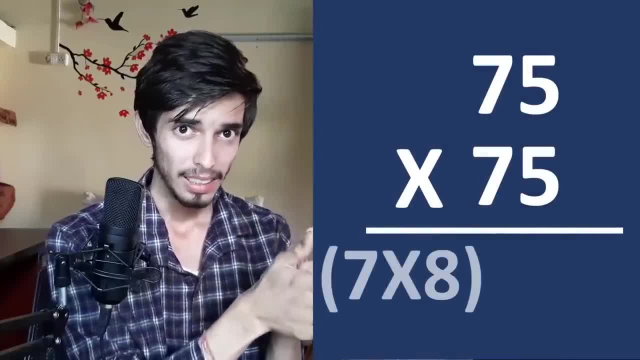 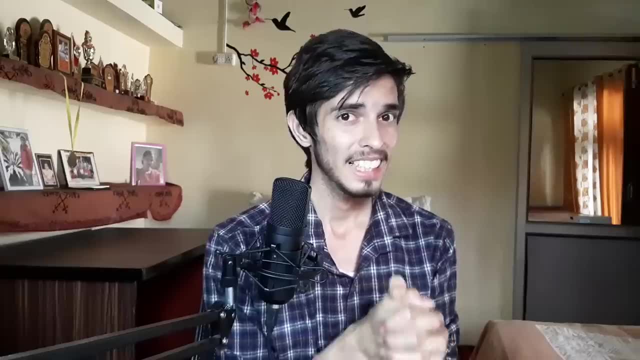 this trick, And the trick is that multiply 7 by its next number, like 7, 8 is a 56 and the answer ends in 25.. So 5,, 6,, 2, 5 is our answer. As simple as that. Let's take some. 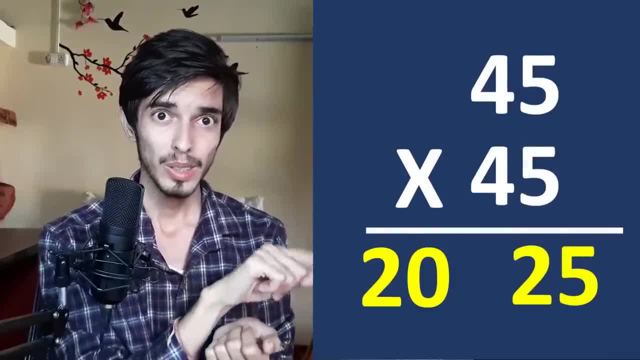 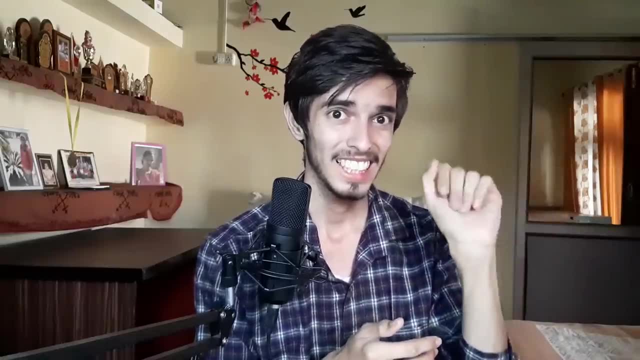 other examples: 45 into 45. So 4, 5 is a 20.. 2, 0,, 2, 5.. 15 multiply by 15.. 1, 2, 0,, 2,, 25.. As simple as that. See, we are faster than a calculator in here also. I just. 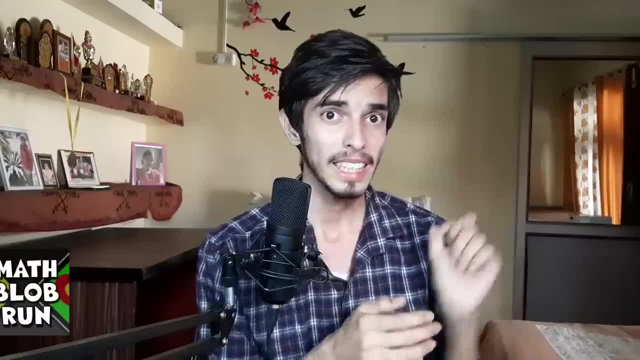 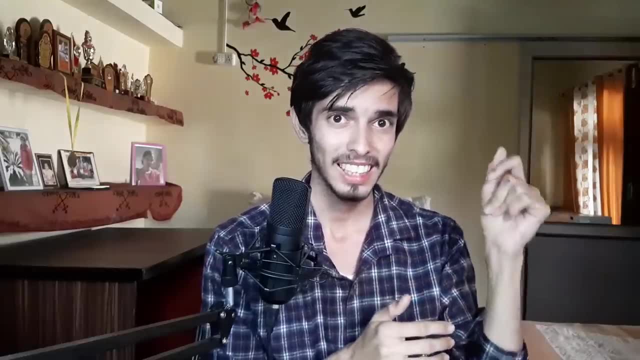 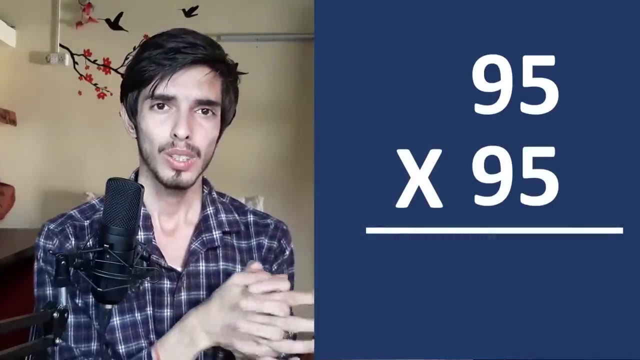 want to tell you that I have added this 75 into 75 problem in my game, Mathlob Run, And people were like, how will we do it in 3 seconds? But here we are doing it in 1 second. Now the biggest number you can do with this trick is 95 into 95.. That is 95 square. So the 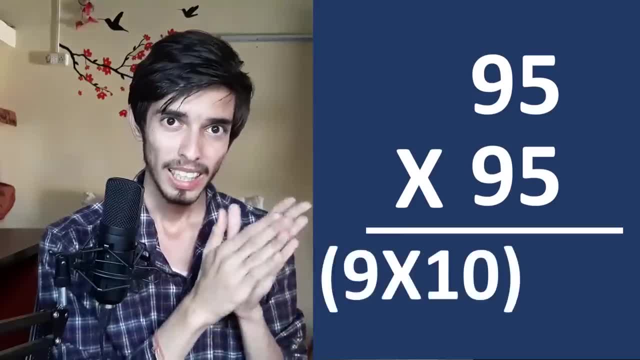 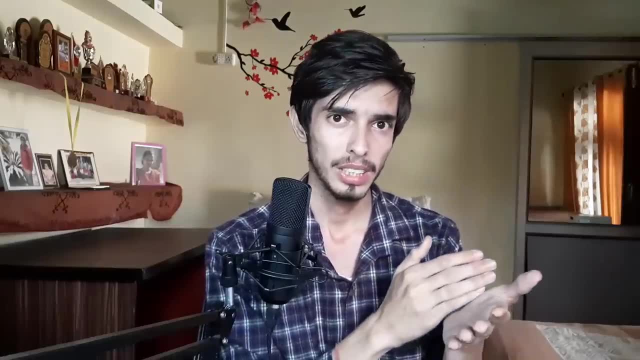 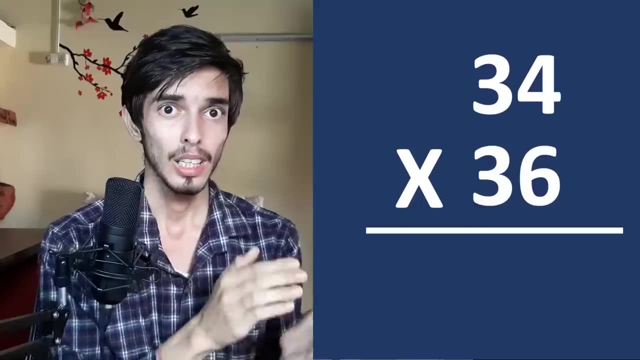 answer is you tell Yes, 9 into 10,, 90,, 25.. As simple as that. We have just done it in a snap. Now this same trick also works with numbers which have same starting digit and the ending digits are adding to 10.. For example, 34 multiply by 36.. 4s are 12 and 6, 4s are 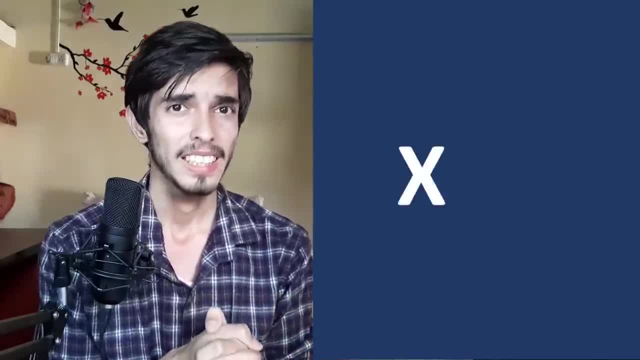 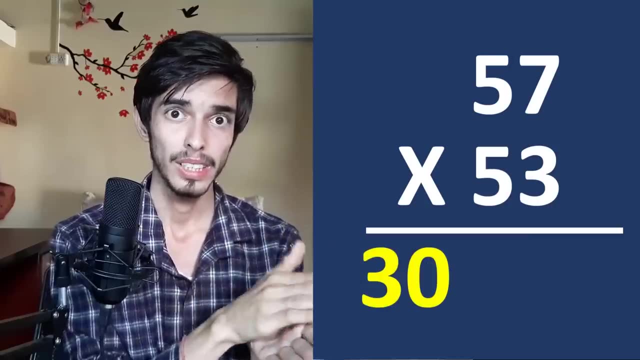 24.. 12, 24 is our answer. So now let's take another example: 57 multiply by 53.. Now you do it. Yes, 6, 5s are 30 and 7s are 21.. 30, 21.. As simple as that. Now, the most important.